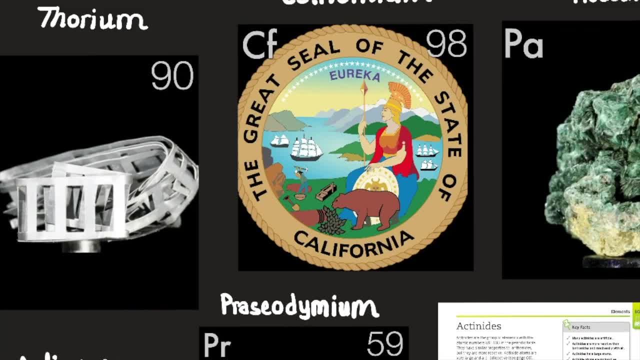 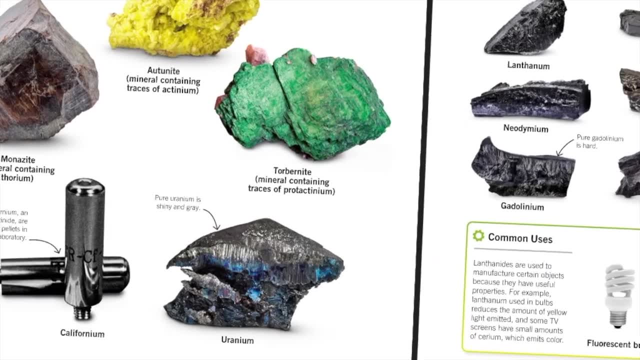 So here we have californium. We don't have an image of it, We have the seal of California. So here we have uranium. Uranium is shiny and gray. Uranium is element number 92. Californium 98.. Here we have torbaronite. 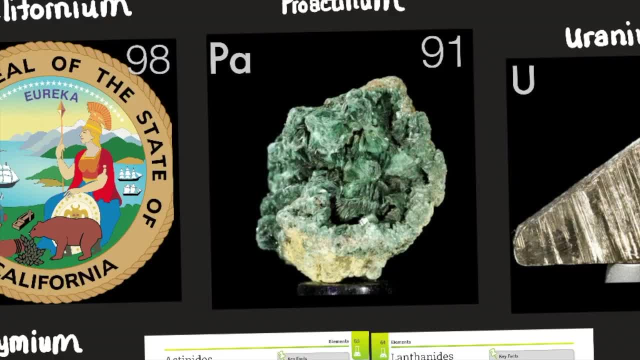 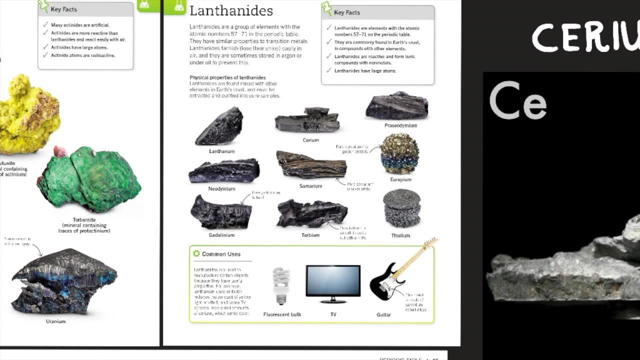 It's a mineral containing traces of proactinium, and proactinium is element number 91.. So we're going to talk about the next group, the lanthanides. Lanthanides are a group of elements with the atomic numbers 51 through 71 in the periodic table. 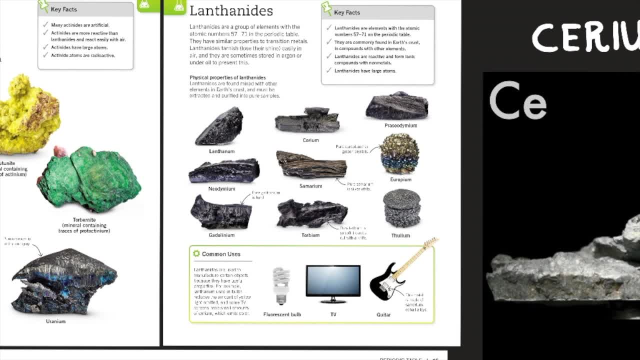 They have similar properties to transition metals. Lanthanides are a group of elements with the atomic numbers 51 through 71 in the periodic table. They have similar properties to transition metals. Lanthanides tarnish. lose their shine easily in air. 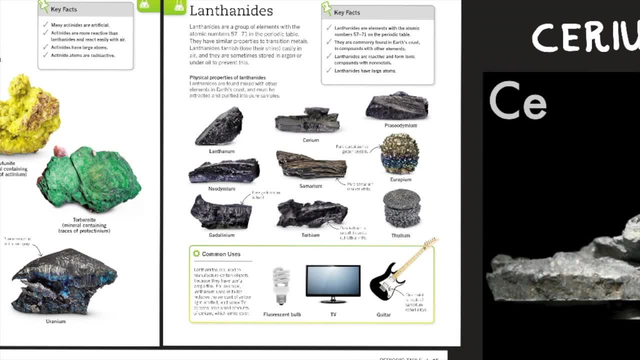 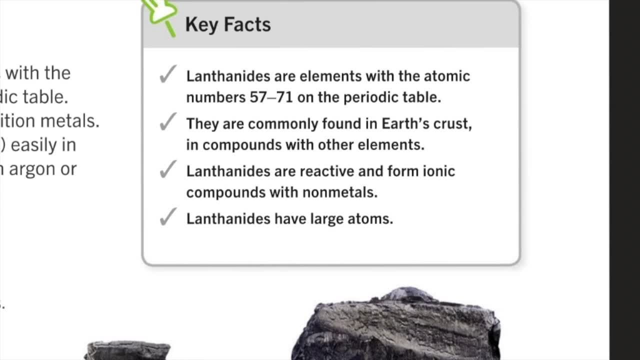 and they are sometimes stored in argon or under oil to prevent this. Physical properties of lanthanides. First key facts: Lanthanides are the elements with the atomic numbers 57 through 71 on the periodic table. They are commonly found in Earth's crust. 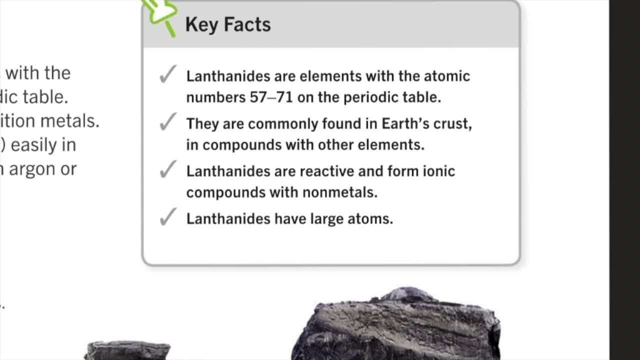 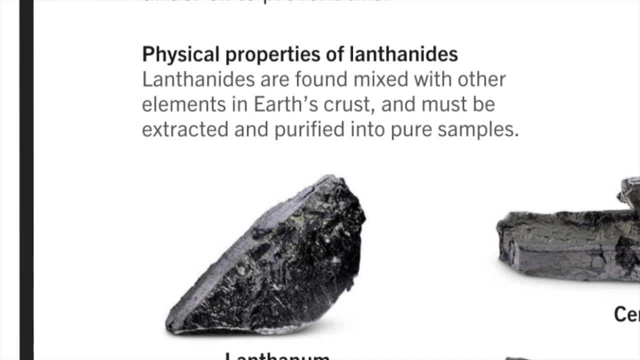 in compounds with other elements. Lanthanides are reactive and form ionic compounds with non-metals. Lanthanides have large atoms. So the physical properties of lanthanides. Lanthanides are found mixed with other elements in the Earth's crust and must be. 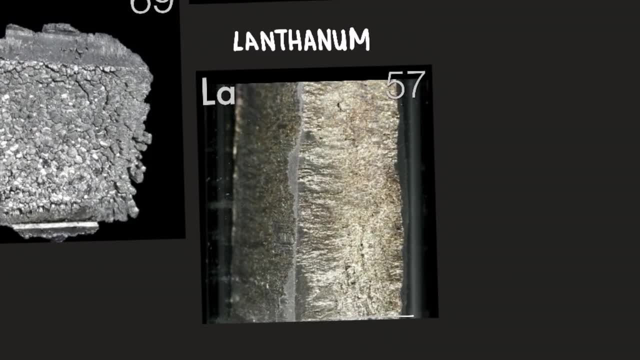 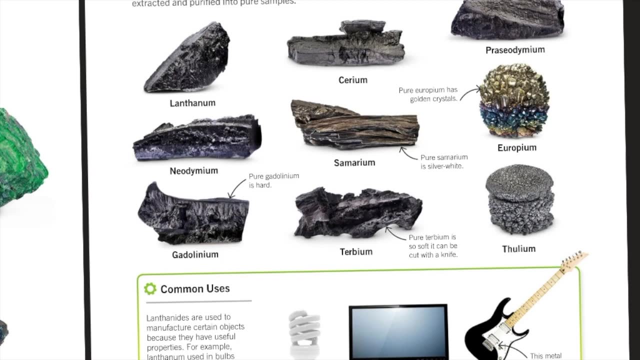 extracted and purified into pure samples. So here we have lanthanum. Lanthanum is element number 57.. And here we have neodymium. Neodymium is element number 60.. Here we have gadolinium. Pure gadolinium is hard. 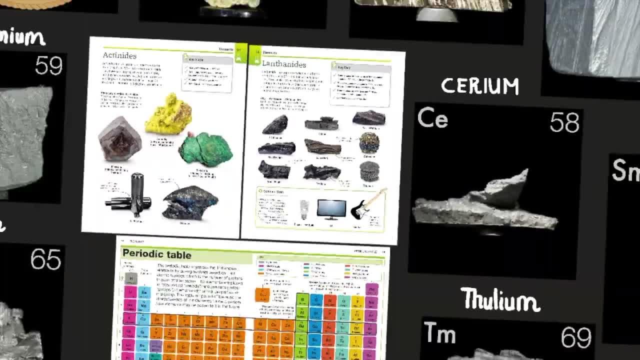 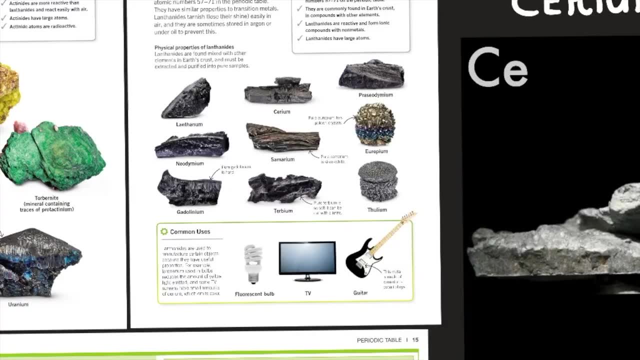 So gadolinium is element number 64.. And here we have cerium. Cerium is element number 58.. And here we have samarium. Samarium is element number 62.. Here we have europium. Europium is element number 63.. 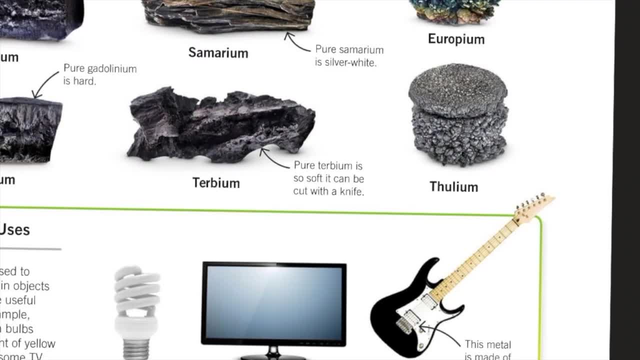 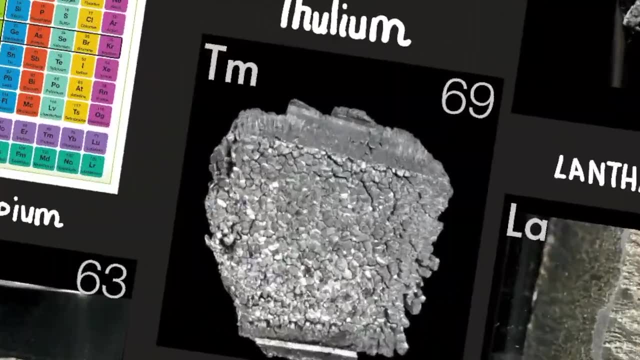 Pure europium has golden crystals. Here we have terbium. Pure terbium is so soft it can be cut with a knife. Terbium is element number 65.. And here we have tholium. Tholium is element number 69.. 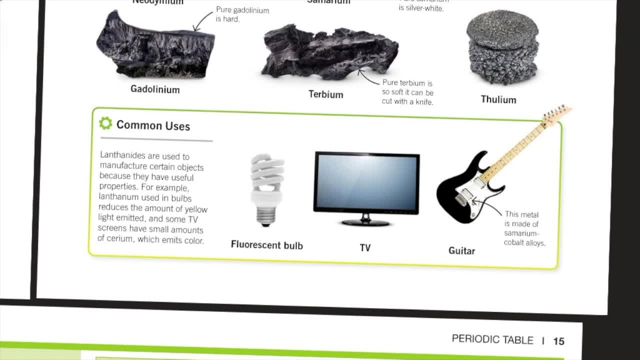 So the common uses of these lanthanides. So what are the lanthanides used for? Lanthanides are used to manufacture certain objects because they have useful properties. For example, lanthanum used in bulbs reduces the amount of yellow light emitted. 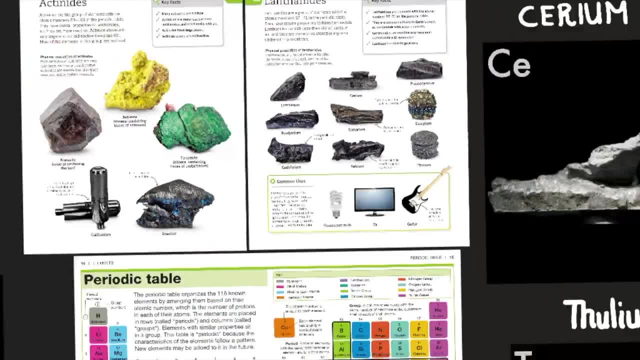 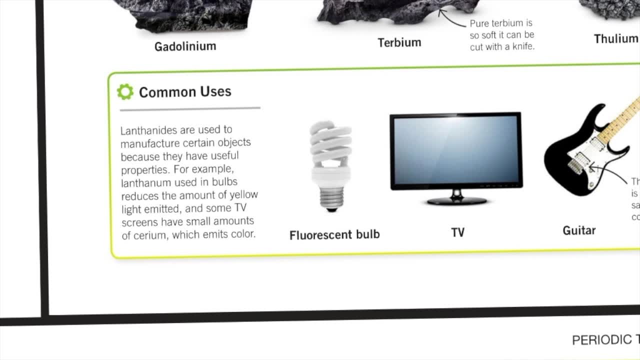 and some TV screens have small amounts of cerium which emits color. So again, cerium is element number 58. So TVs use element number 58 in small amounts because it emits color, which is useful for the TV. Here we have fluorescent bulbs, TVs and guitars.